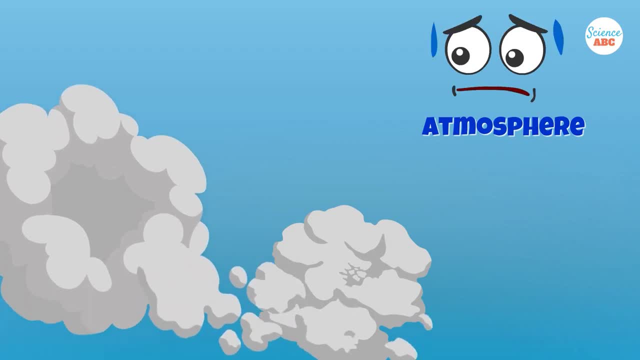 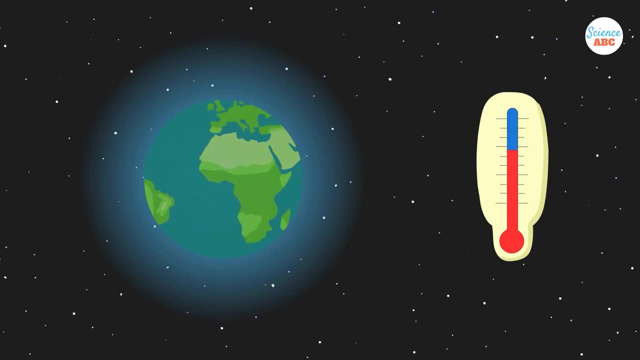 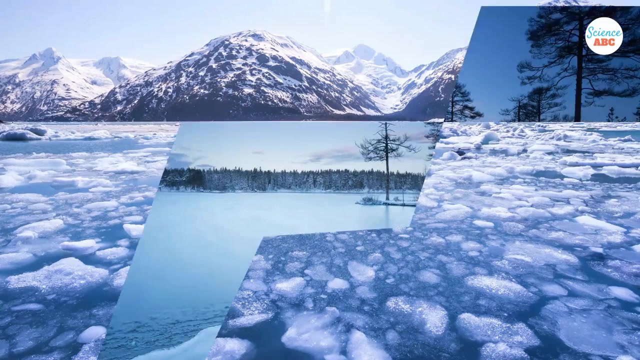 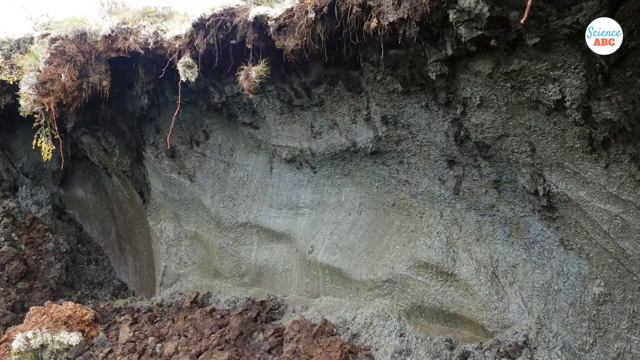 This is why rising carbon dioxide emissions is a point of great concern to every nation on the planet. The rise in global temperature changes several other weather patterns and geographical conditions. For example, the climate of the United States is changing as the weather changes. The climate of the United States is changing as the weather of the United States changes. For example, the climate of the United States is changing as the weather of the United For example, an increase in temperature directly impacts the snow, river, and lake ice, sea ice, glaciers, ice caps, ice shelves, and ice sheets, as well as frozen ground, also known as permafrost. The rising surface temperature causes a decline in ice mass. 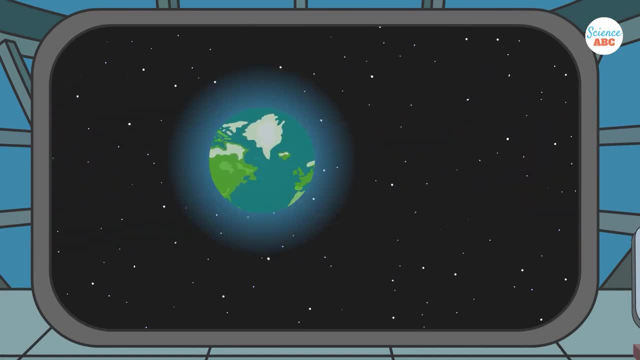 Ice mass measurement by NASA's satellite shows that the Antarctic and Greenland mass is declining at an unprecedented rate. 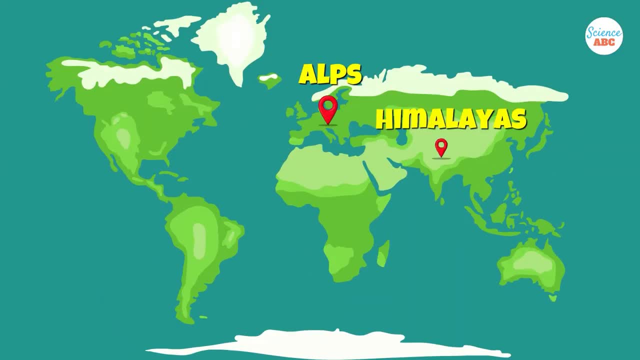 Glaciers are also retreating almost everywhere, including the Alps, Himalayas, Andes, Rockies, Alaska, and Africa. 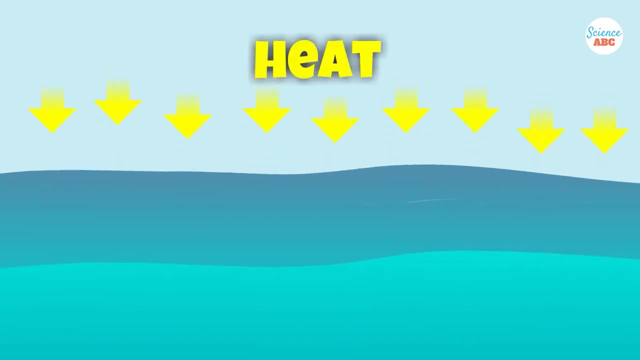 Furthermore, oceans absorb almost 90% of the excess heat from the surrounding air, making it warmer. 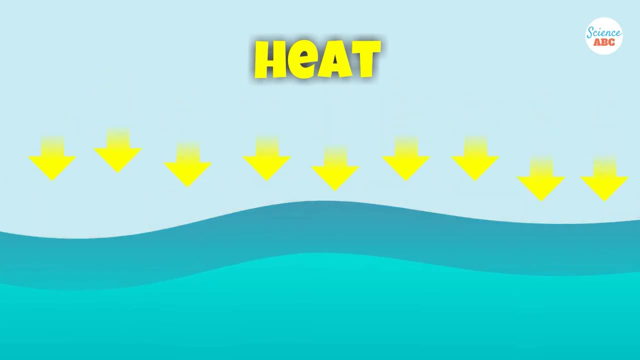 Although most of the heat is absorbed in the surface as the rate of warming increases, the heat permeates to deeper waters and harms marine ecosystems. 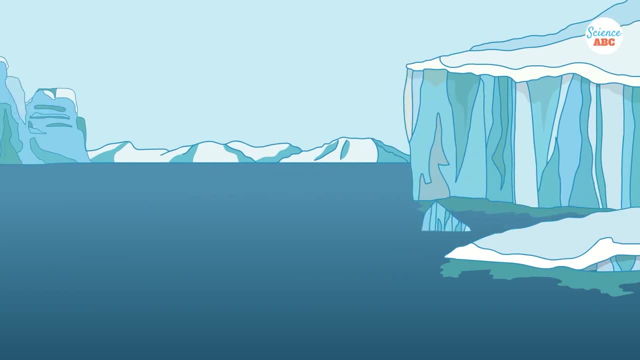 Sea level rise is caused primarily by water from melting ice sheets and glaciers, and the expansion of seawater as it warms. 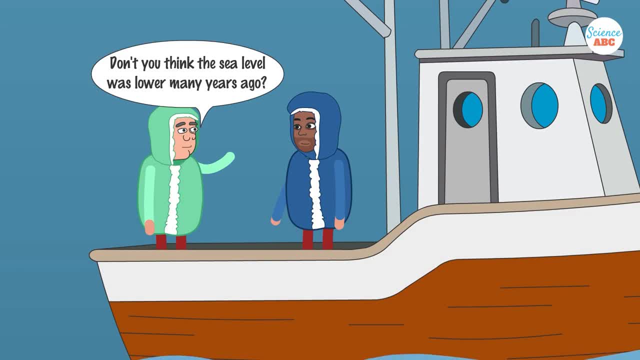 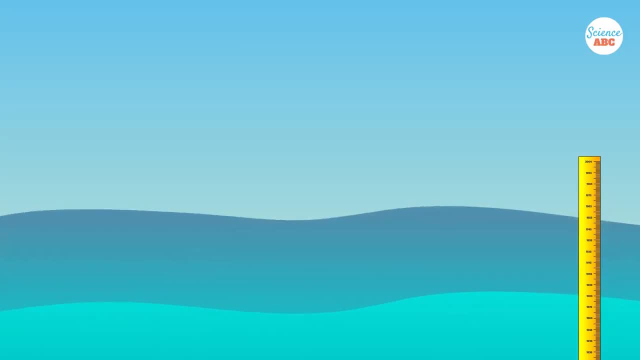 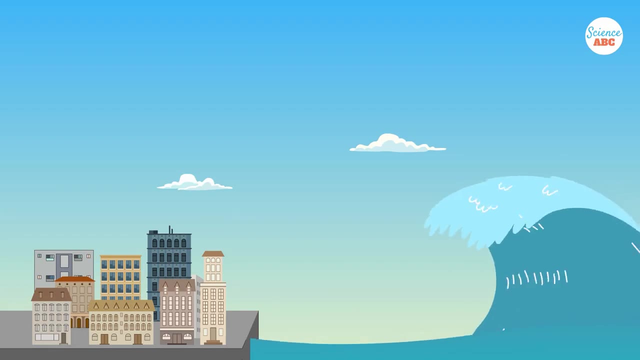 Satellite observations indicate that the sea height is increasing rapidly. The rise in sea levels negatively affects the populace of coastal areas. It also plays a role in flooding and leads to an increase in storms. Climate change also leads to changes in the frequency, intensity, spatial extent, duration, 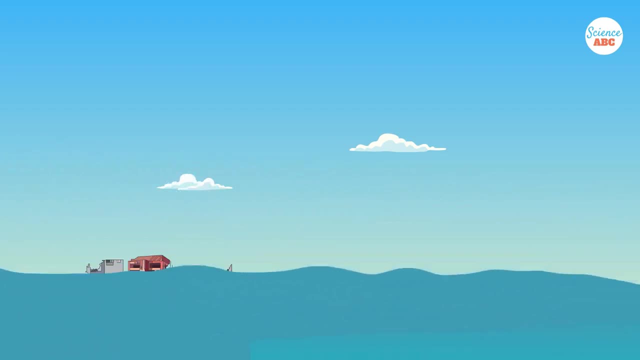 and timing of weather and climate extremes. Some extreme weather events include floods, droughts, hurricanes, and heat waves. 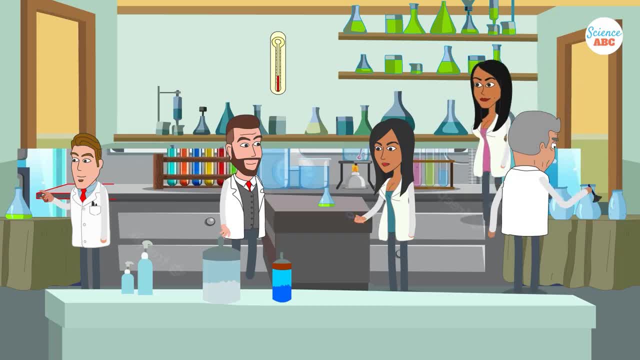 Weather and climate extremes occur when the weather or climate conditions are not in the same order. 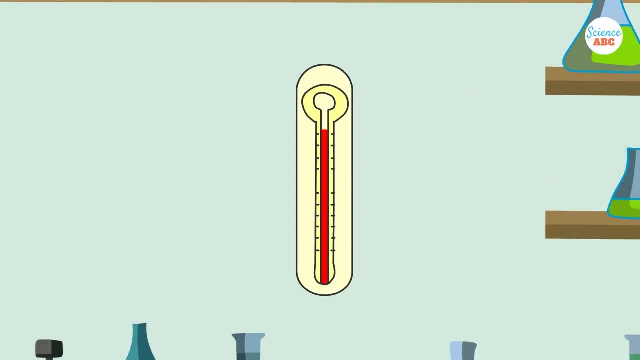 Weather or climate metric is above or below a threshold value of the variable. 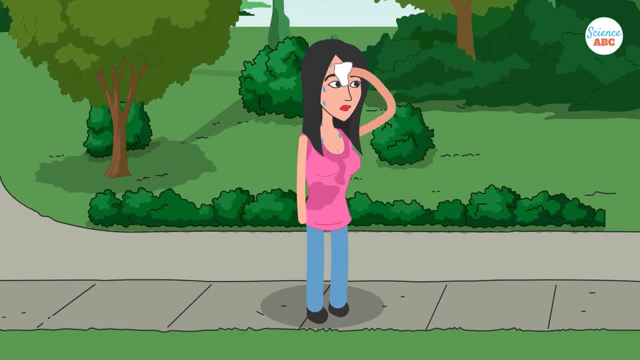 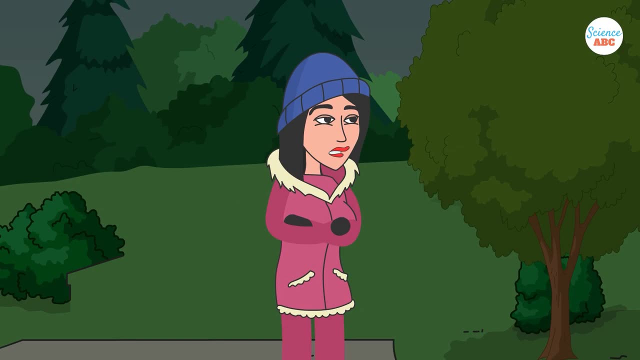 Some of the changes in weather patterns include an increase in the number of warm days and nights, a decrease in cold days and nights, and an increase in the frequency and intensity of daily temperature extremes.